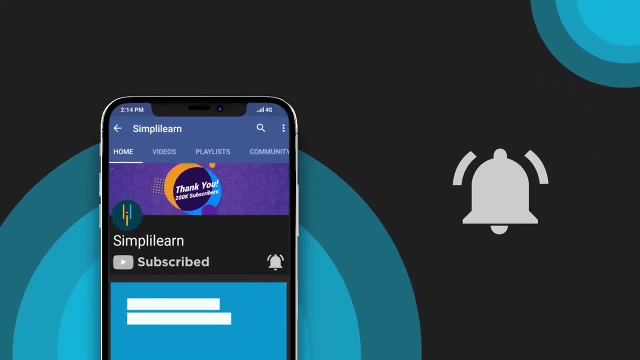 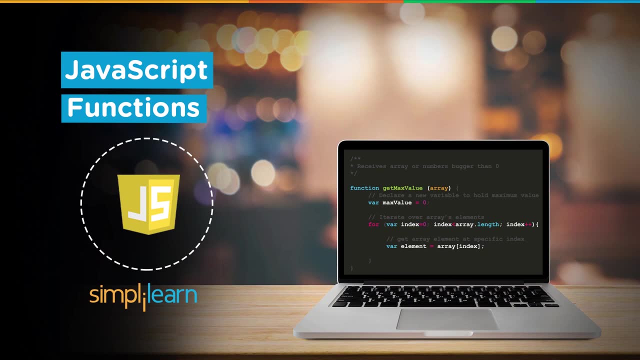 Hey guys, welcome back to another video by Simply Learn. In today's video, we're going to learn all about JavaScript functions. In our previous videos, we've covered topics like JavaScript arrays and loops. If you're new to this topic, I suggest you go through. 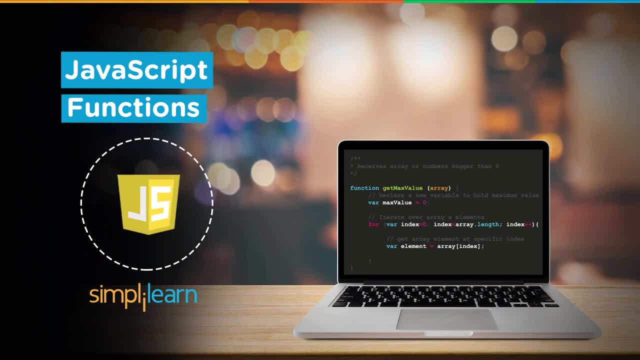 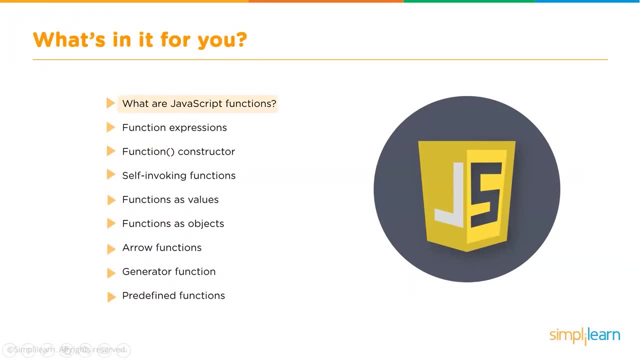 these topics before. Alright, so before jumping in, let's go ahead and look at what's in store for us. First we're going to learn what exactly JavaScript functions are, Then we'll look at JavaScript function expressions, then the function constructor self-invoking. 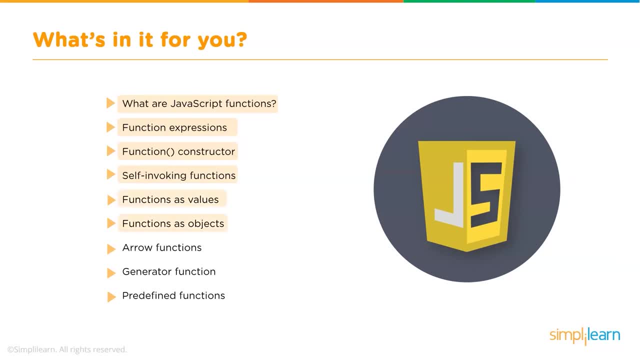 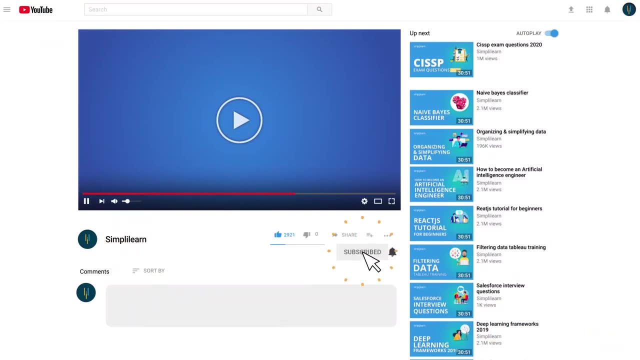 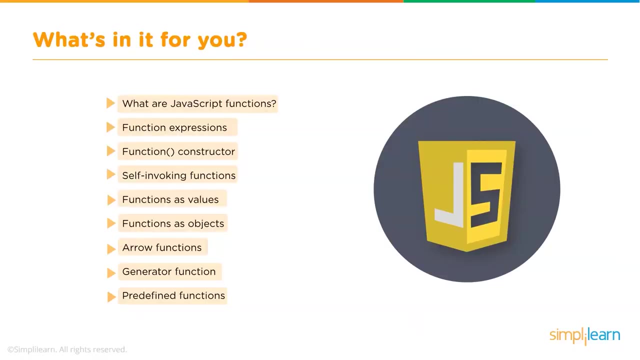 functions: functions as values, functions as objects, arrow functions, generator function and the predefined functions. Also, don't forget to subscribe to our channel and hit the bell icon to never miss an update. Moving on to our first topic, what are JavaScript? 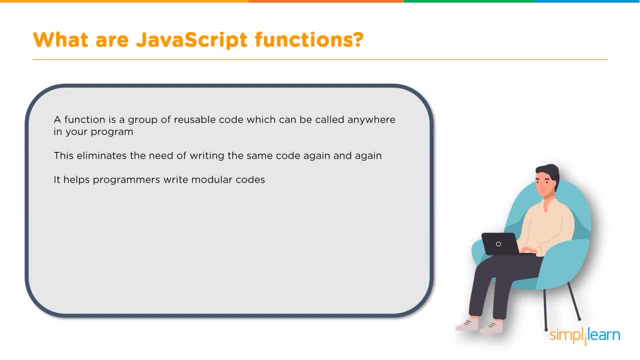 functions. So basically, a function is a group of reusable code which can be called from anywhere in your program. right, When you have a piece of code that you want to execute repeatedly in your entire program, it makes more sense to define it once and 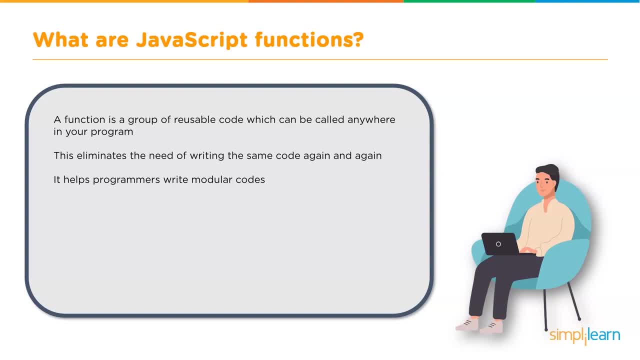 call it over and over right. It makes the code more efficient and readable. This also helps programmers write modular codes. So this is the syntax: You make use of the function keyword, followed by which you make use of the function keyword, followed by which you 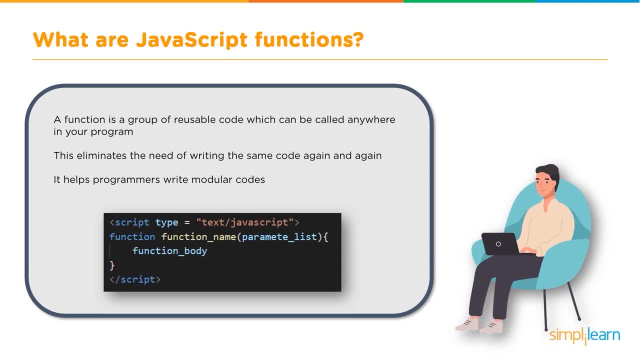 make use of the function keyword, followed by which you make use of the function keyword, And then you mention the name of the function. The name of the function is completely your choice. Next, you mention the parameter list And within curly braces, you can define the. 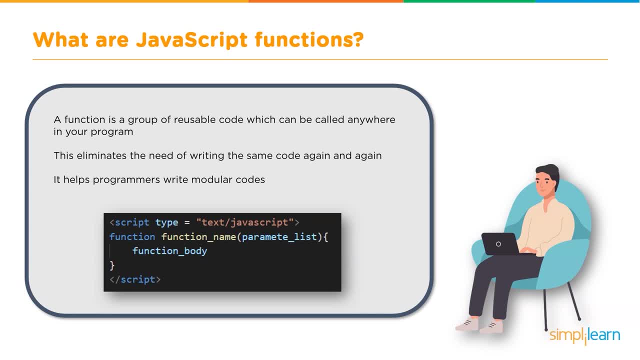 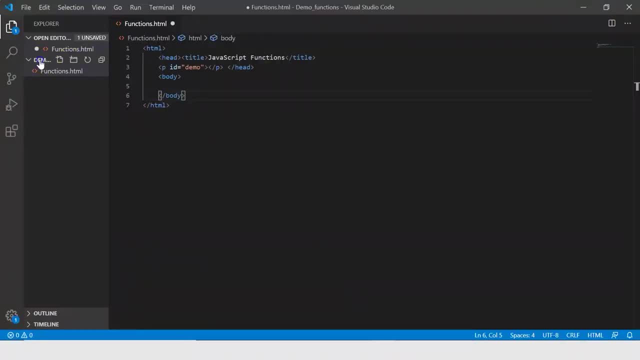 function. Now the function body is basically the code that is executed every time the function is called. So let's go to our VSCode editor, And here I've created a folder called demo functions, within which I've created an HTML file called functionshtml. All right, And 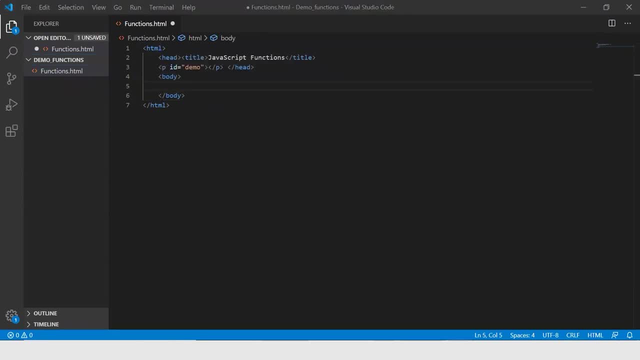 now I've just typed in the initial code. Now let's create a function. So let me say script, within which I use the keyword, that is function keyword. And now I give the name for my function, I say my underscore function, and the function takes a parameter, say value. 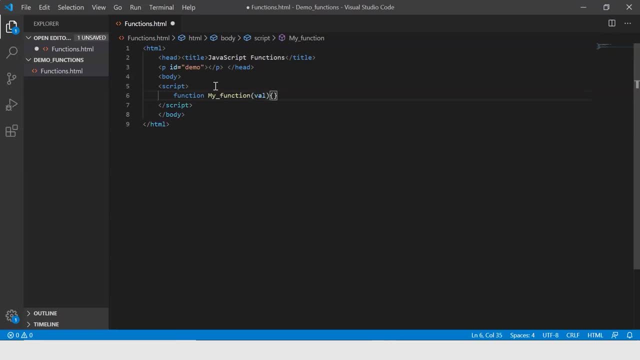 Now this function basically returns the square of the digit right So, within which I say documentgetElementById, the ID is demo, And now it just displays value into value. all right, So the function basically displays the square of the number. Now, outside the function, let me call the function. it is my function and let me pass. 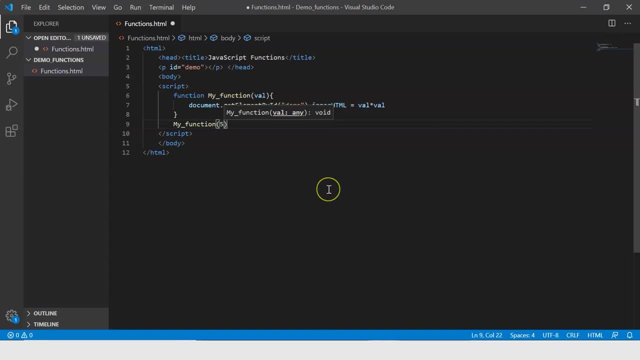 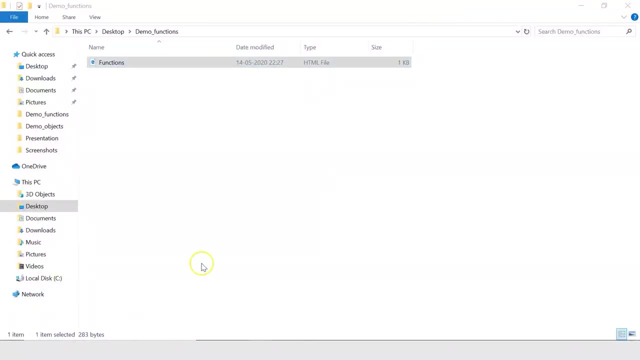 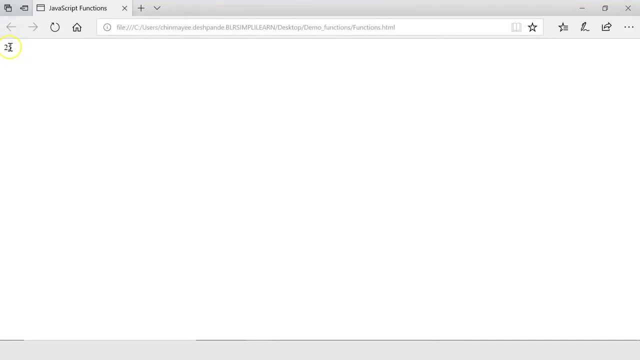 the function. It displays the value 5,. all right, Now let's save this and execute it. So let me go back to my file and here we go: it displays the value 25.. So this was a simple function which took a value, a digit, as a parameter and then returned. 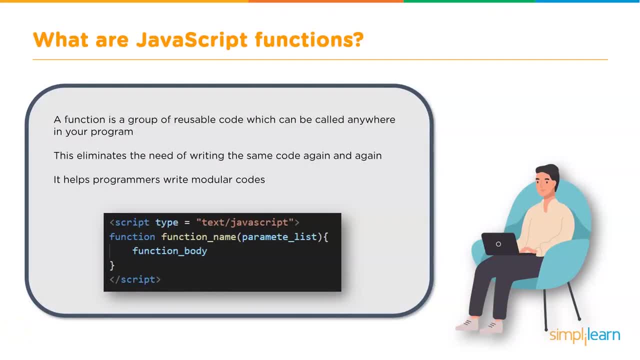 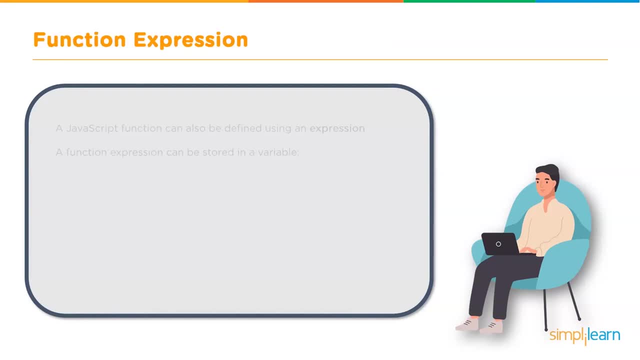 the square. Moving on to the next concept: function expression. Now, what we learned previously was function declaration, but a function can also be defined as an expression. Now, this is what the syntax looks like. Now, here the function is created and assigned to the variable explicitly, like any other. 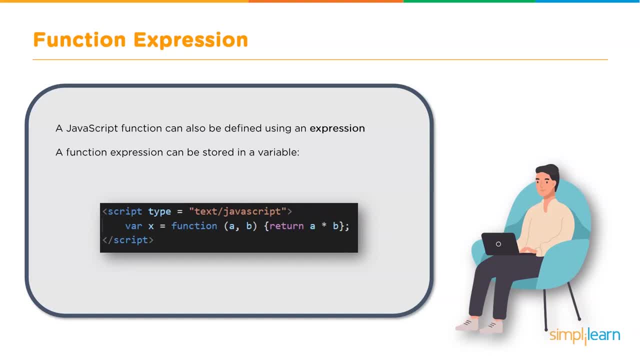 value, The meaning remains the same, that is, you create the function and store the value that it returns into a variable, and in our case it's x, right? So let's go to our VS code and let me help you understand this better. 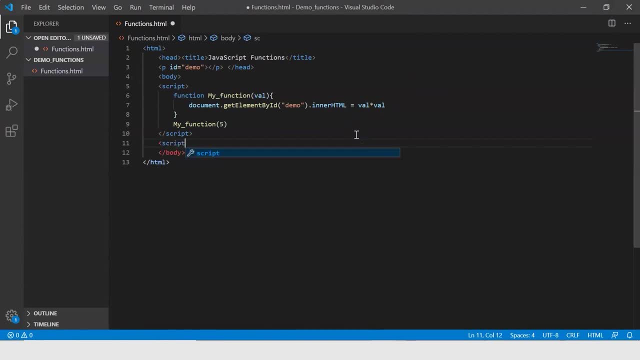 So now I create another function and here I say: let x equals, let's use a simpler function. So I just mention function and within curly braces I display an alert message and I display a message saying hello, all right. Now, after that, to display the message, what we can do is 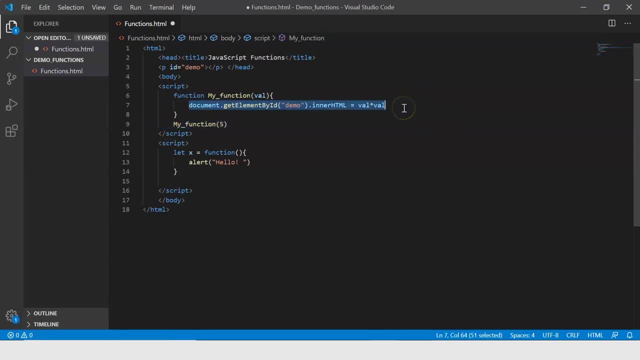 Let me just copy this output code and paste it here and here. what we're going to be displaying is the value x right Now. since it consists of a function, you'll have to type the curly braces Now. this is crucial for its execution. all right, 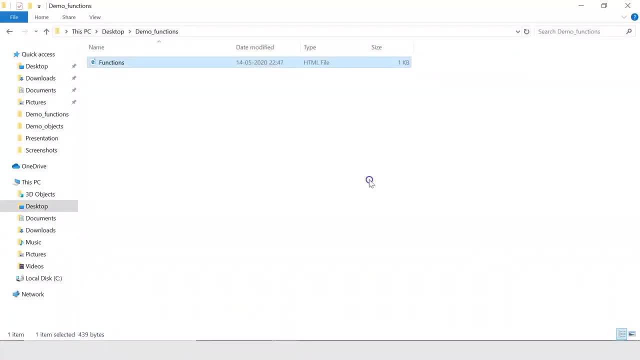 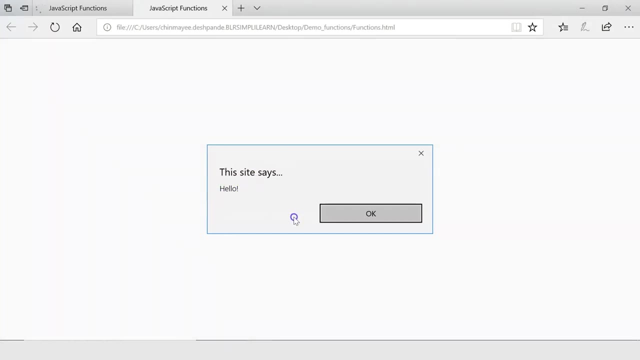 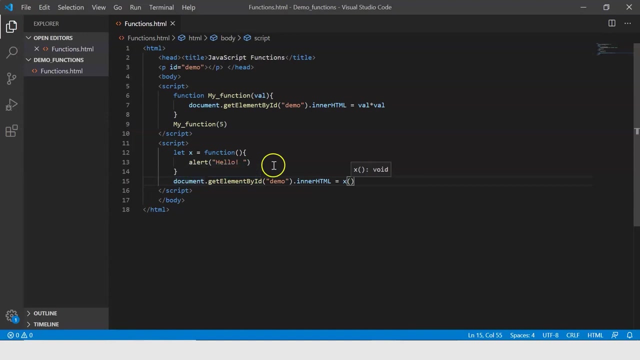 So let me save this and then execute. Let me execute this and here you go. It says the site says hello. So we've successfully executed the piece of code. We can also assign this variable x to another variable and then call that variable instead. 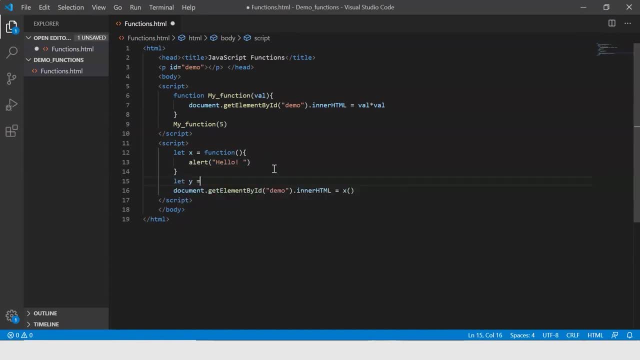 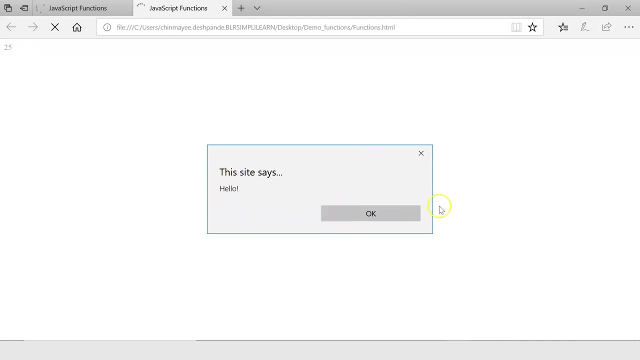 right, We can say: let y equals x, and instead of calling x here, we can simply call y. Let me save it, and then let me refresh the page. and there we go. It still displays the message: hello, All right. So this is one of the ways of defining a function. 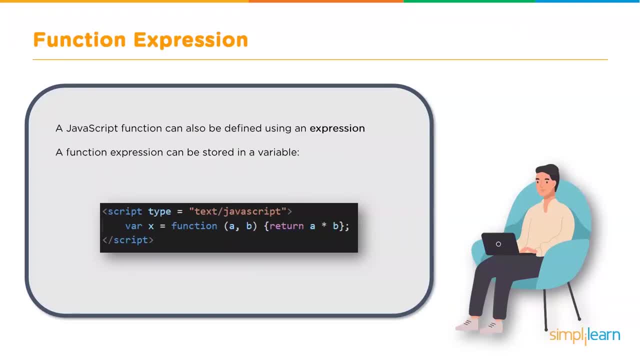 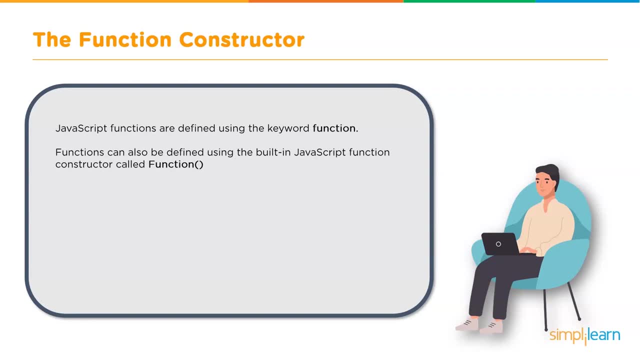 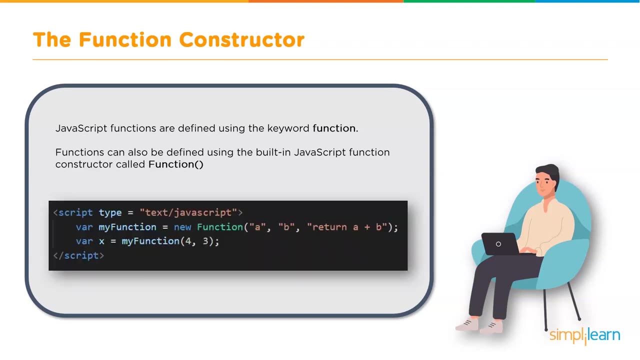 That is as an expression. Moving on to our next concept: function constructor. Now, JavaScript functions are defined using the keyword function. right Now, functions can also be defined using a JavaScript built-in function. Now, this is the basic syntax. So here we've created a function called my function and we've used the keyword new. 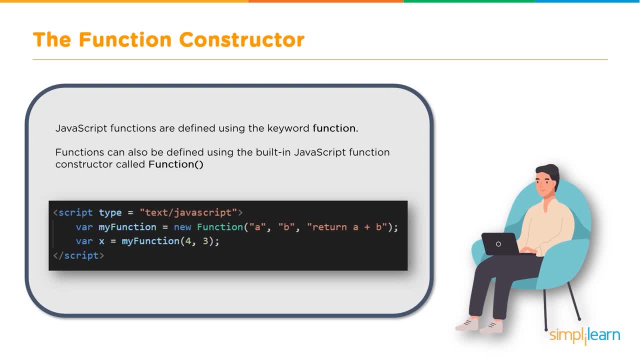 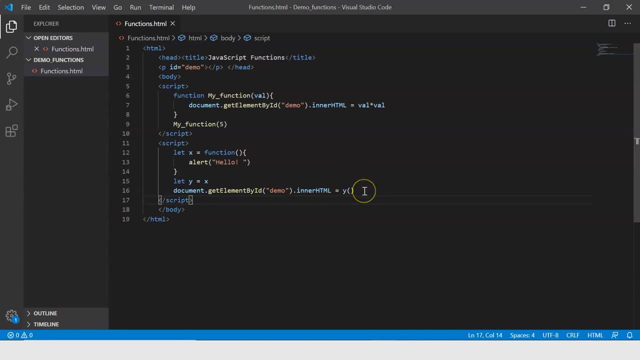 After which we've used the constructor function and inside we provide the parameter list, After that the return value. All right. Next, you can call the function here, right? So let me just go back to my VS code. and now let me just make changes to the same piece. 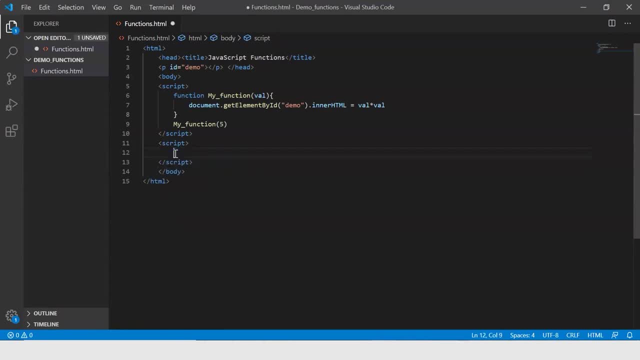 of code. here I create a function, say my underscore function. Okay, All right, Let me just change the name to my function, All right. And then here I use the keyword new and the function constructor, that is, function, within which I'm passing all the parameters. 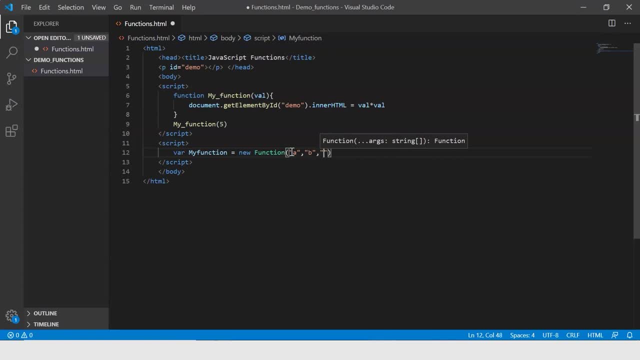 So I have AB and I'm going to return the sum of the digits. All right, And now, while calling the function, let me just store the value in a variable, say x, And then I'm going to return the sum of the digits. 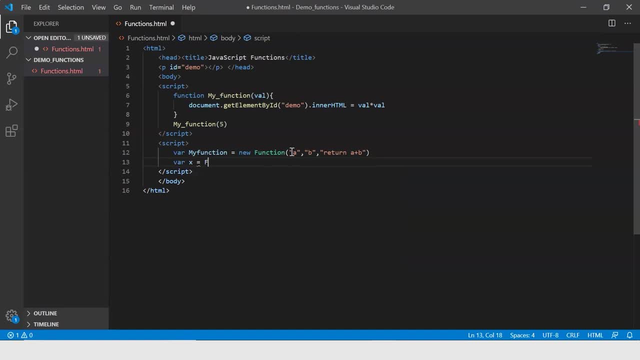 All right, And now, while calling the function, let me just store the value in a variable, say x, And let's call the function- that is my function- with the parameters two and three. All right, And now let me display it. So I'm just going to copy this and I want to display the value of x, right? 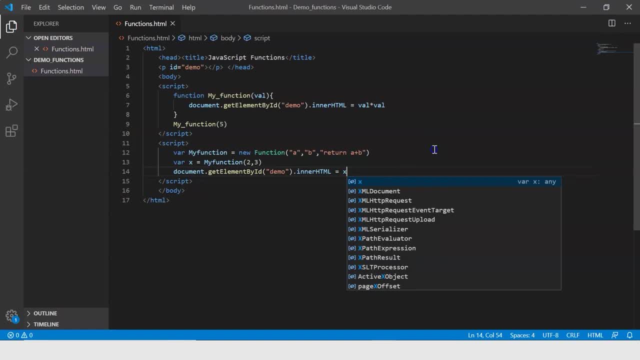 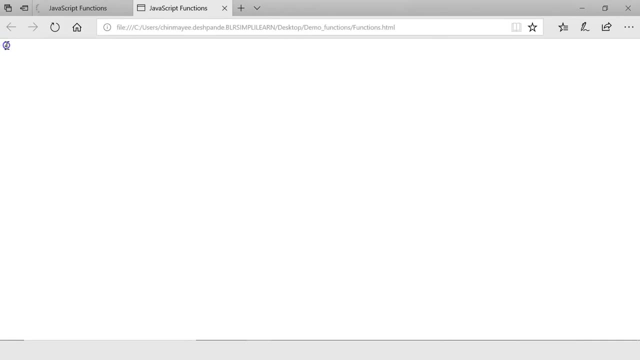 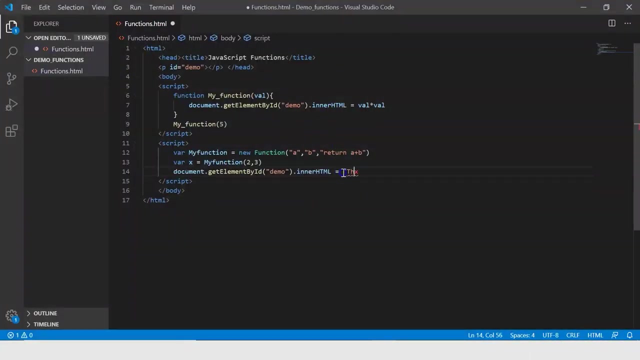 All right, So let me save this and execute it. Okay, If you refresh the page, it displays the sum, that is five. To make it more readable, let me just display another message here. Let me just say the sum is x. 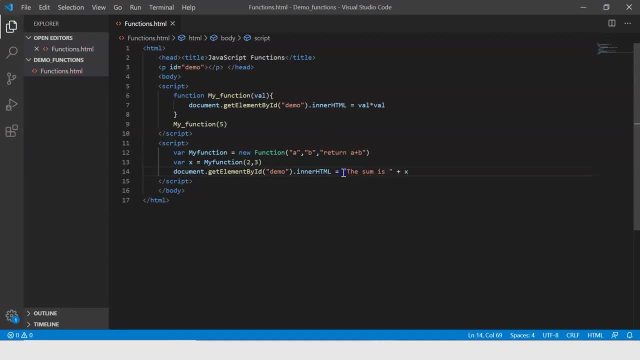 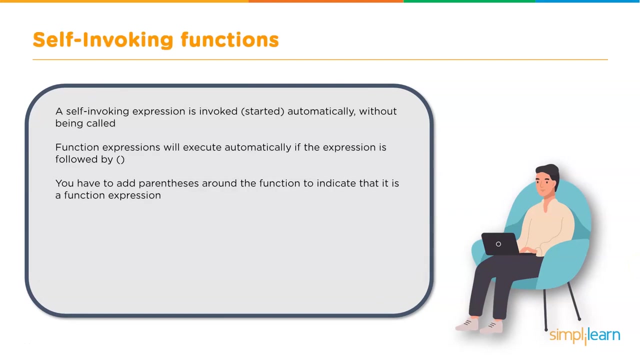 All right, Let me save it and then refresh the page. it says the sum is five. All right, Now this is how you make use of the function constructor. Next up, we learn about self-invoking functions. Okay, Now, as the name suggests, these functions are invoked automatically without being called. 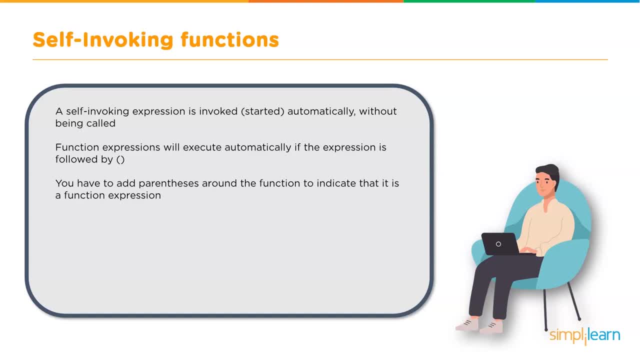 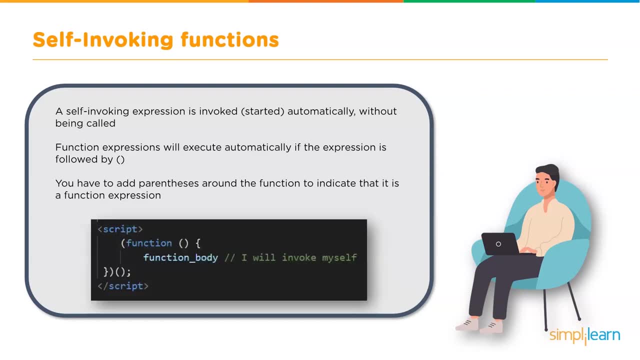 Now, previously, when we learned about function expressions, we saw that parentheses were crucial. So you have to add parentheses around the function to indicate that it is a function expression. So here is a syntax for you. So what we've done is we've made sure we've enclosed the entire function within parentheses. 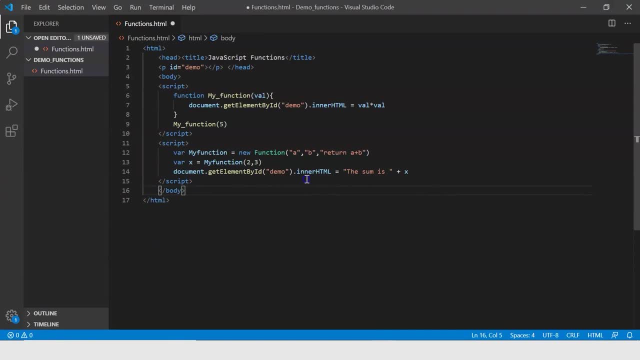 So let me help you with that. Let's go back to our VS code And let me show you how to do that. So let's go back to our VS code And let me create another script, And here let me create the function within the parentheses and say function. 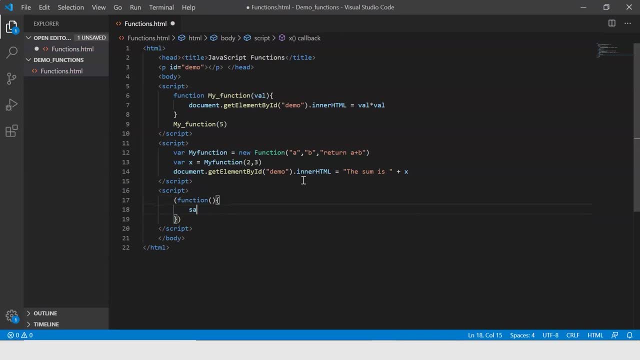 It's not taking any parameters. Instead, it is going to alert a message. So let me say hello, welcome, All right, After which we're going to call the function. So again, we have to mention the parentheses, All right. 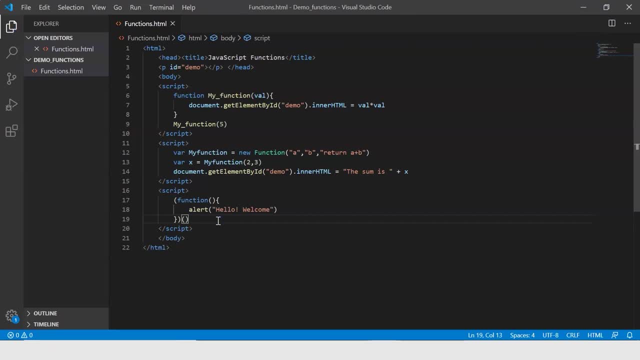 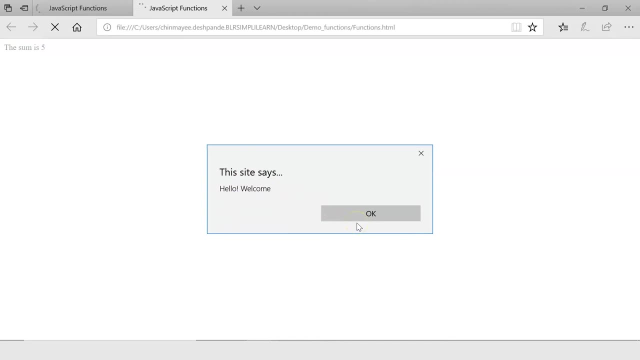 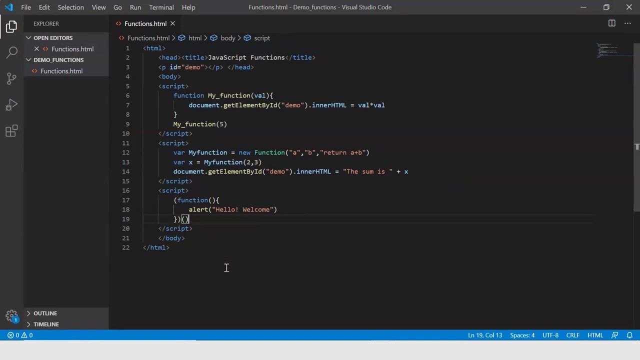 Let's save this and execute. So when we refresh the page it says hello, welcome. So we never call the function, rather, it got invoked by itself. So these are self-invoking functions. Now let's go ahead and look at functions as values. 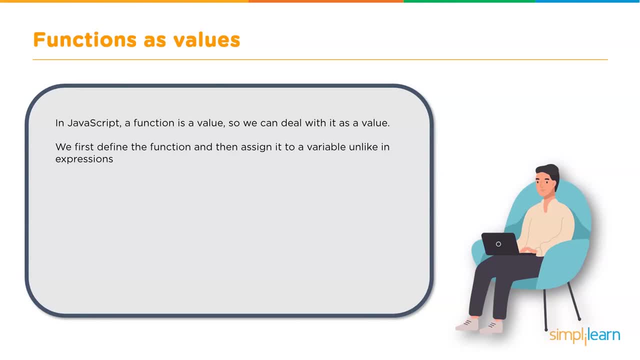 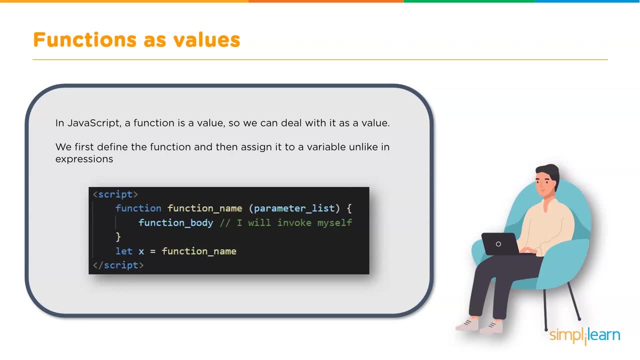 Now, in JavaScript, a function is basically a value, So we can deal with it as a value. Now here is a simple syntax. Now, if you closely look at the syntax, you might think that this is same as function expressions. Well, no. 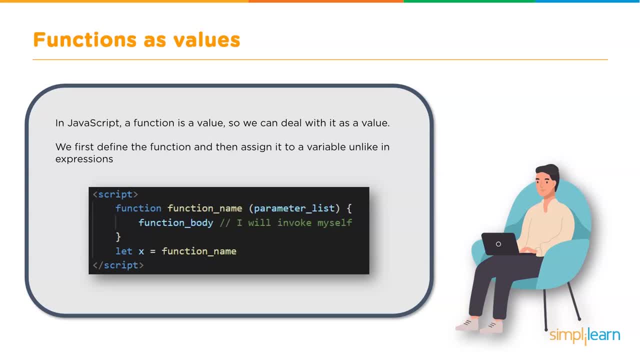 In this case, what we do is we first define the function and then we assign it to a particular variable. But in the case of expressions, the function definition was defined during the initialization of the variable Right, And also we have to specify the parentheses in order to call the function. 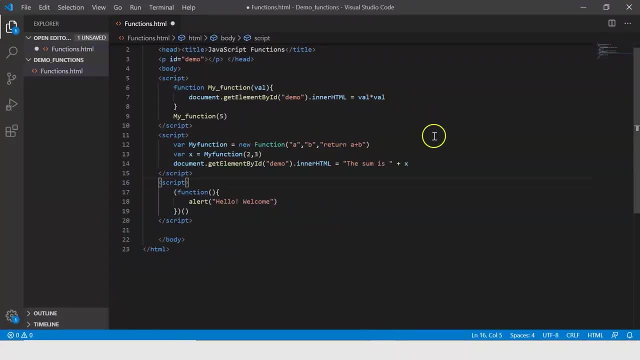 So, to help you understand this better, let me go back to our VS code, All right, And here let me just erase this and let's define a function that returns the product of two digits. So let me just call it product, which takes two parameters, let me say a and b within. 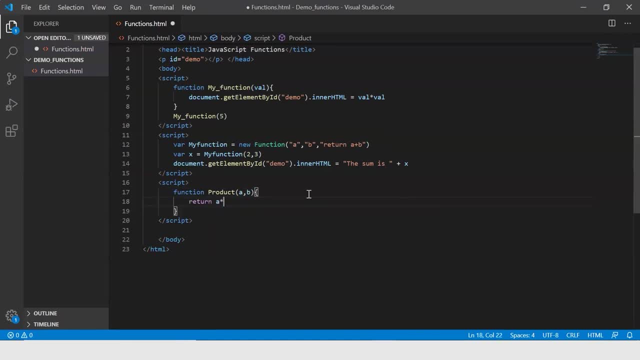 which we return the value a into b. All right Now, after this, let's create another variable say y. So let's create another variable say y. All right Now, after this, let's create another variable say y. 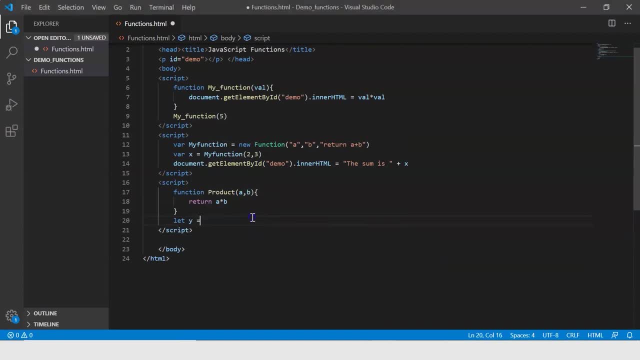 All right. Now, after this, let's create another variable, say y. All right, So product equals function. oh, I'm sorry, the name of the function is product, so product of two and five, Right. So this basically returns us 10, right? 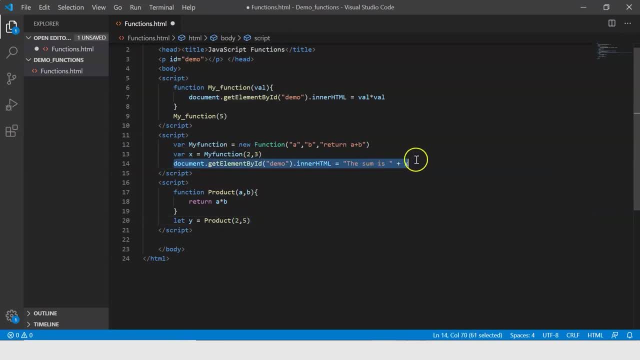 So let me just copy this to display this on our webpage, And here I'll change the message to the product, And here let me change it to y. So let's save this and execute it. So here let's write the message. 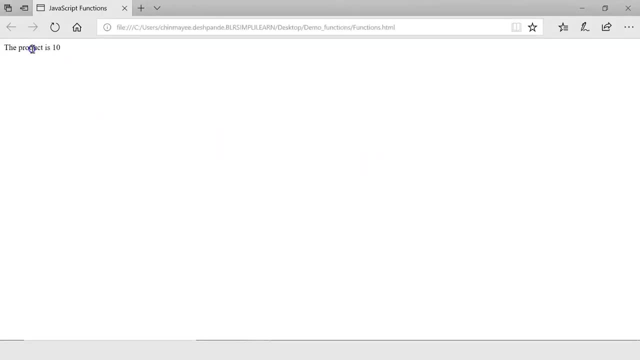 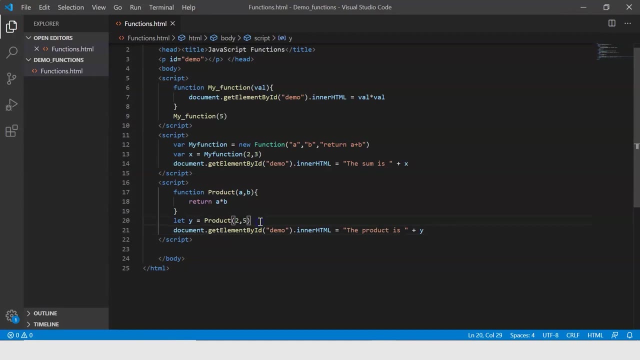 so let me refresh the page. and here you go. you can see the message. the product is 10. now what we can do is we can make alterations to this. now say, I want to multiply the value with 5 again, right? so basically, this returns 10 and that value 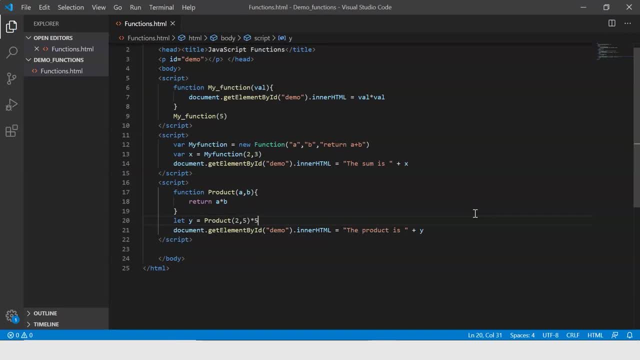 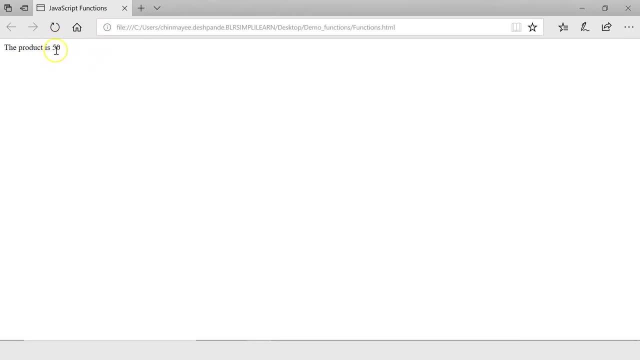 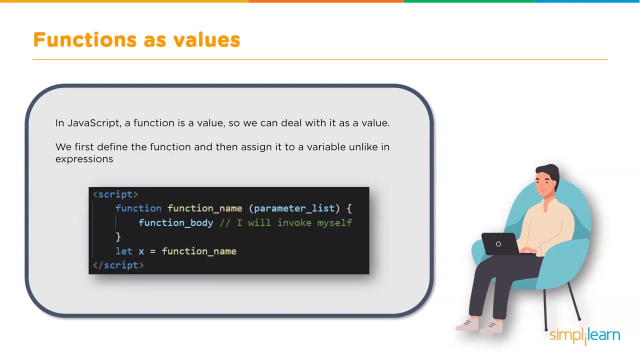 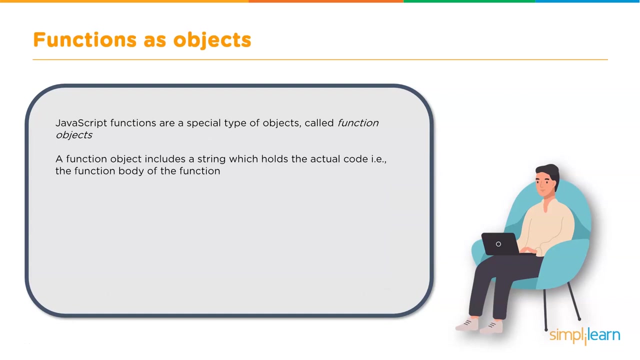 is multiplied by 5. so let me save this and refresh our page. and there we go, it returns. and there we go, it displays 50. so this is how you can make use of functions as values. moving on to the next topic: functions as objects. now JavaScript. functions are a special type of objects called function objects, now a. 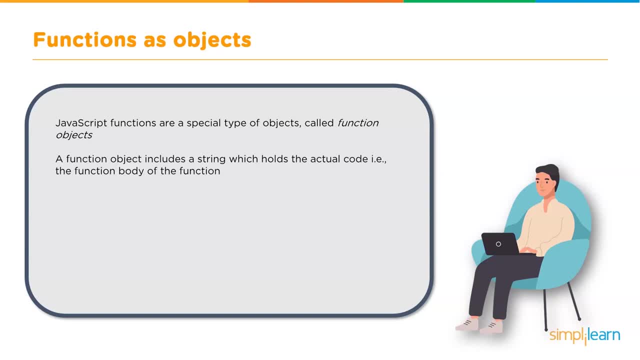 function includes a string which holds the actual code. that is, the function body of the function. the code is literally just a string, although not recommended. you can also create a function body of the function. the code is literally just a string, although not recommended. you can also create a. 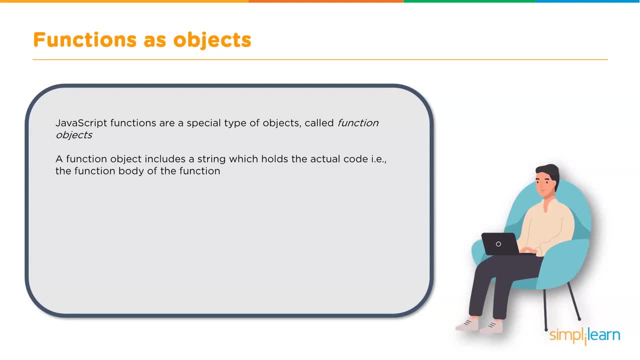 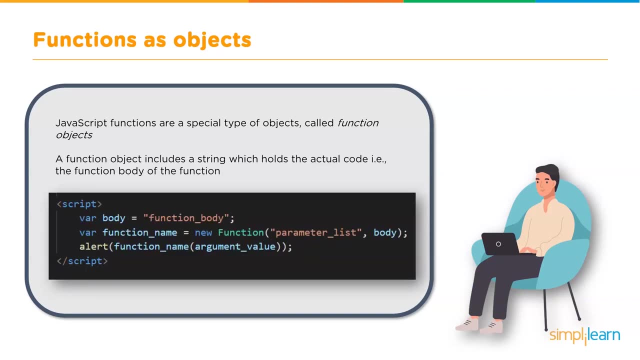 function with the help of the function constructor. I will show that you a little later on, but for now let's look at the syntax. now here we have a variable called body, which basically consists of the function body. it's enclosed in double quotes and that's a mistake. please ignore it, alright? so next, 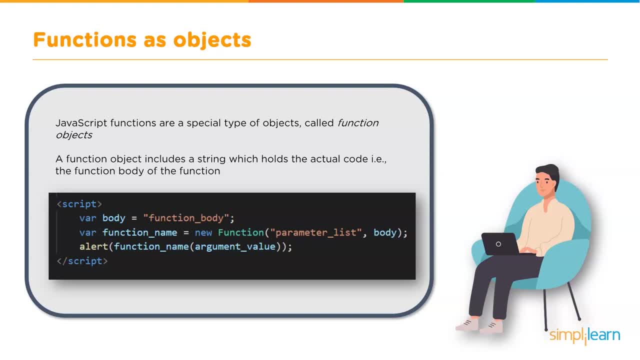 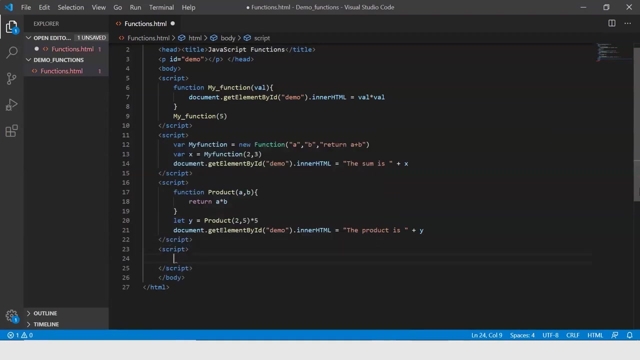 we have variable function name. so here we create a function using the keyword new and then we pass a parameter list and the body basically tells us what the function returns. right next we have an alert message to call the function. so let me just show how this is executed back in our VS code. let me create another function and let's say: 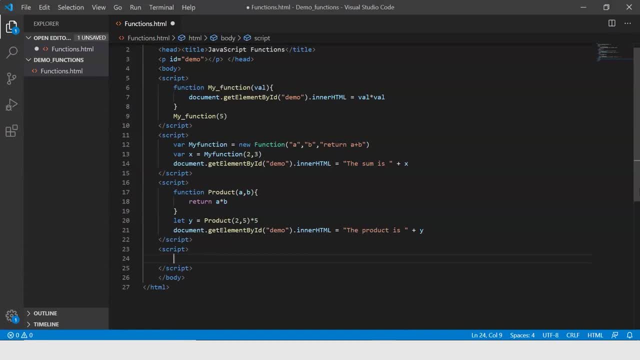 the function returns the area of a circle, right. so let me just create a body variable which returns. so the area of the circle is pi R square. so we make use of matpi into radius. into radius is right, so is basically by our square. after which let's say battel. 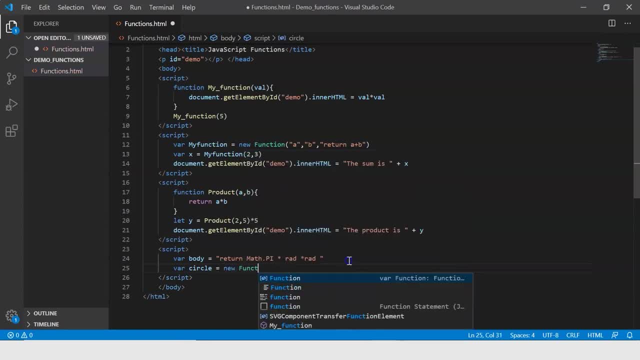 and here let's create a function using the new keyword function, and here will pass the value, that is, the radius and and then the body, right. So basically, this is the definition of our function. So let's use alert to display the area. 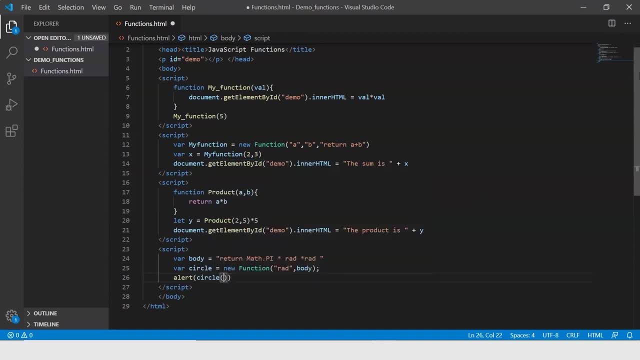 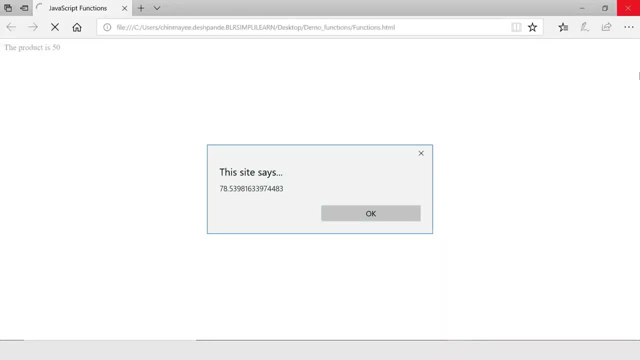 So we say: alert of circle of five. All right, let me save this and execute it. So when you refresh the page it displays the area of the circle. So this is how you can use functions as objects. Moving on to our next concept, arrow functions. 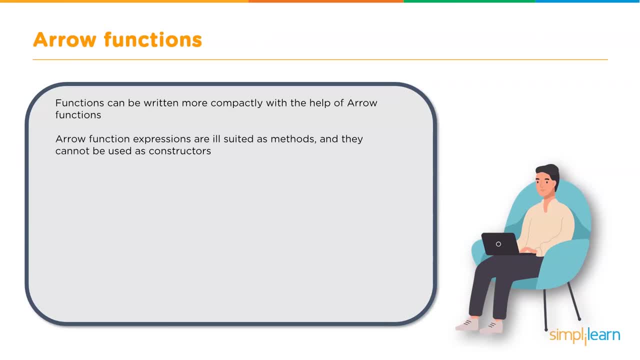 Now, functions can be written more compactly and more precisely with the help of arrow functions. All right now. arrow function expressions are ill-suited as methods and they cannot be used as constructors. Now also, while using arrow functions, using const is a safer option. 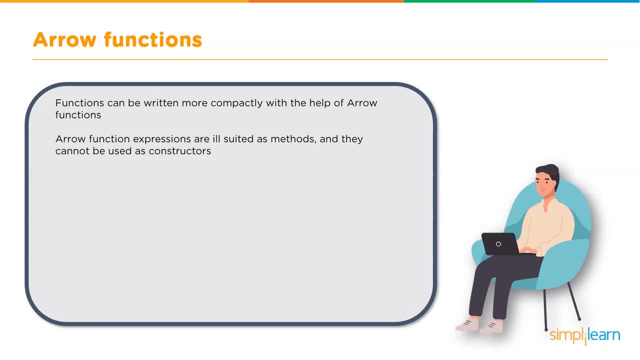 because a function expression is always a constant value. So this is the syntax. Now you can only omit the return keyword within the curly braces if the function is a single statement. So this is the syntax. First, you provide the name of the function with an equal to sign, followed by the argument list. 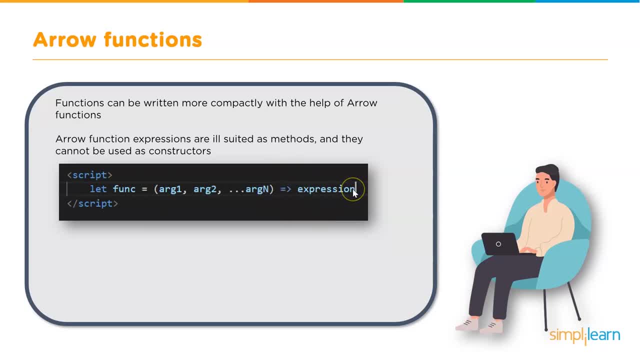 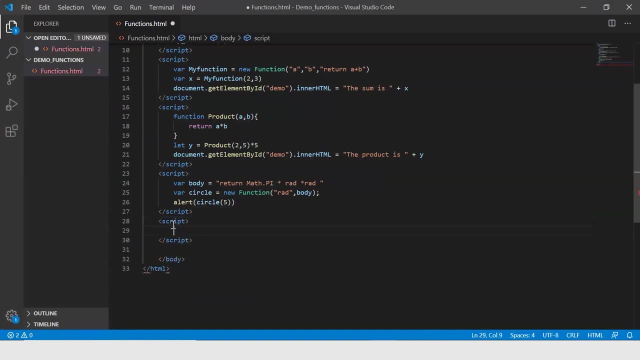 And later you make use of this arrow icon and define the expression. So this is basically nothing but this. So let's go back to our VS Code and check for ourselves. So let's create another function, And here let me say: const myFunk equals. 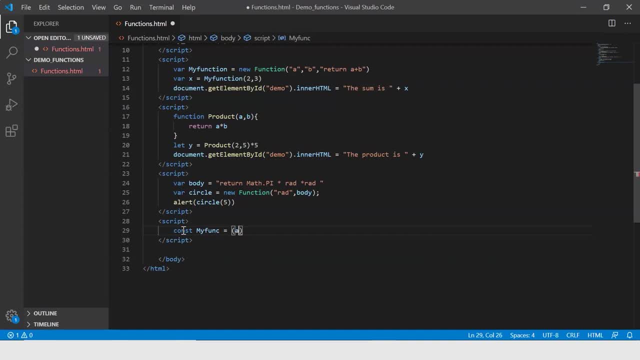 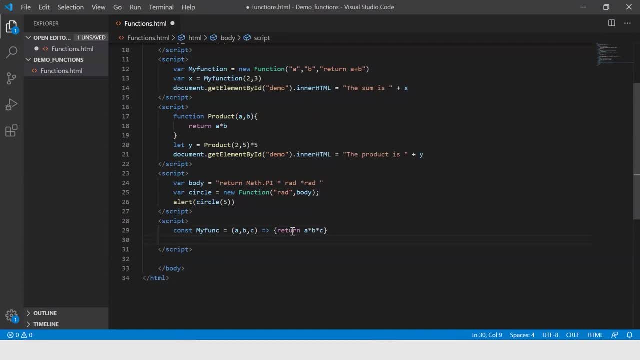 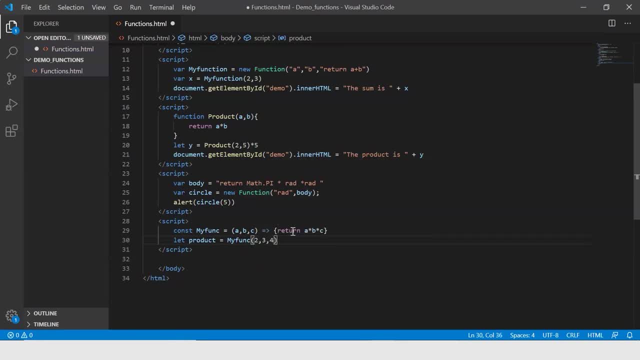 and pass the value two, three and say four. All right, so let's display the product. So let me just copy this. All right, so let's display the product Code. And here let me say the product of the three digits is: 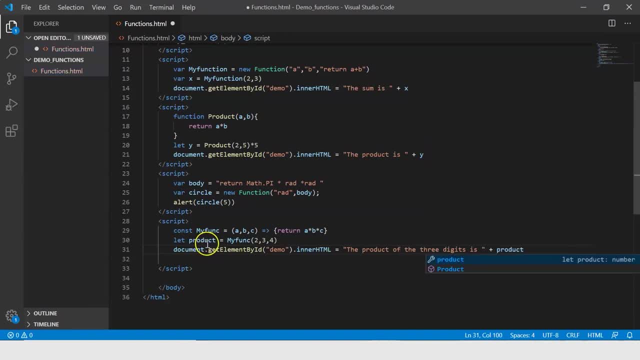 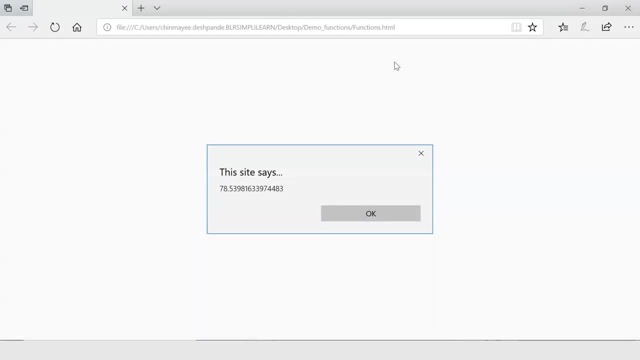 And let me say product here, because that is what is being used here- right, All right. so let me save this and execute it, All right. first it displays the area of the code. All right. first it displays the area of the code. 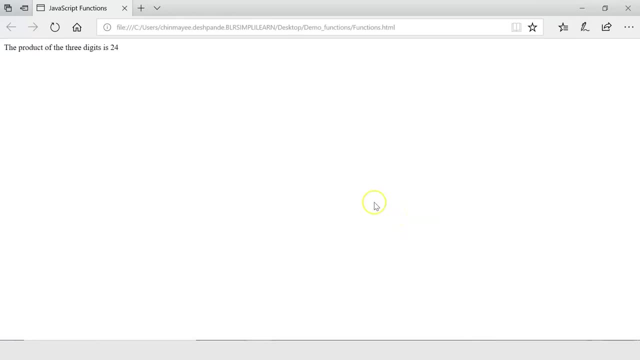 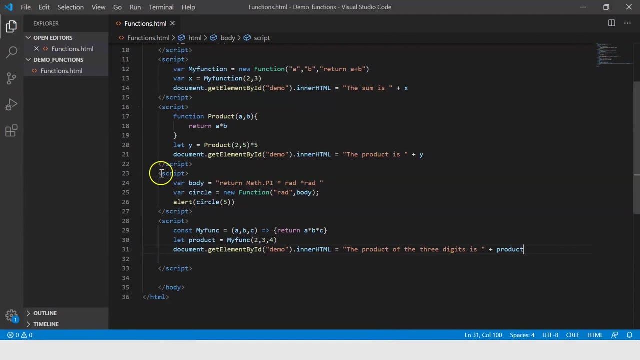 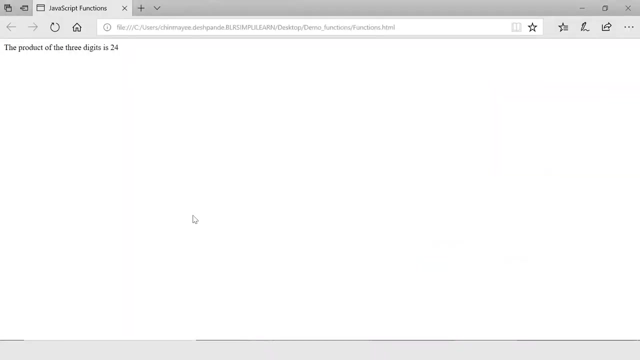 It's a circle, All right, and then we say okay, And there we go. It displays the message: the product of the three digits is 24.. So let me do one thing. Let me just comment this out. Okay, Let me save it and then execute it again. 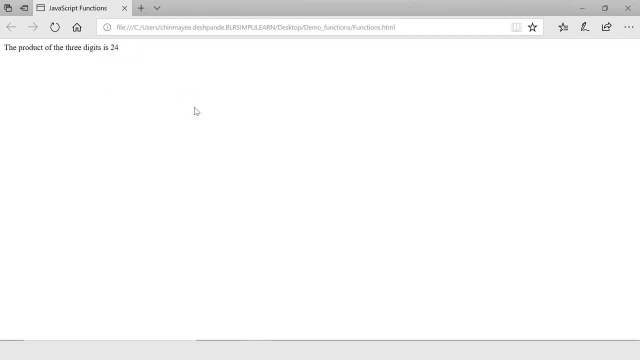 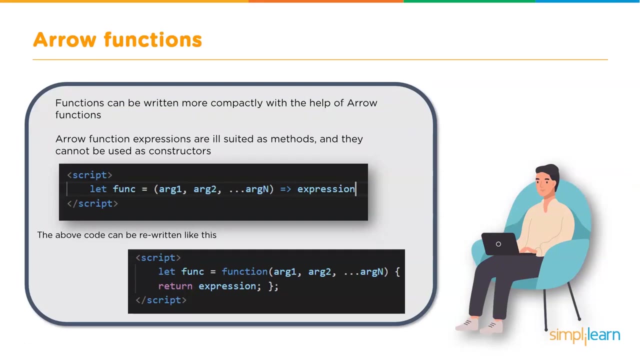 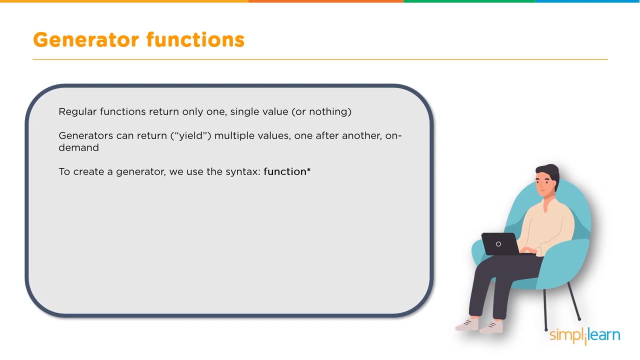 It just displays this. All right, so this is how we can make use of arrow functions. Moving on, let's look at the generator function Now. regular functions typically return only one value right, Or a single value, Or sometimes even nothing. 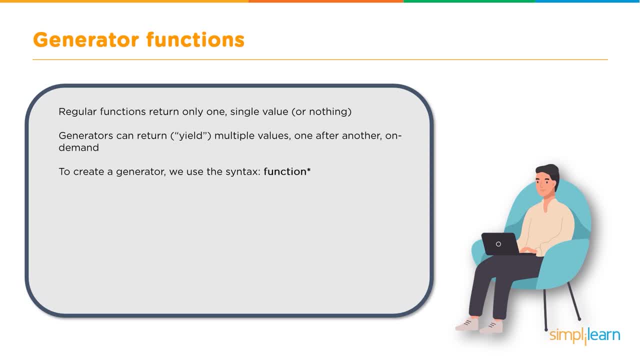 But a generator function can return multiple values And the speciality is that it can do it. so on demand, All right now to create a generator function. we make use of an asterisk, So an asterisk indicates that the function is a generator function. 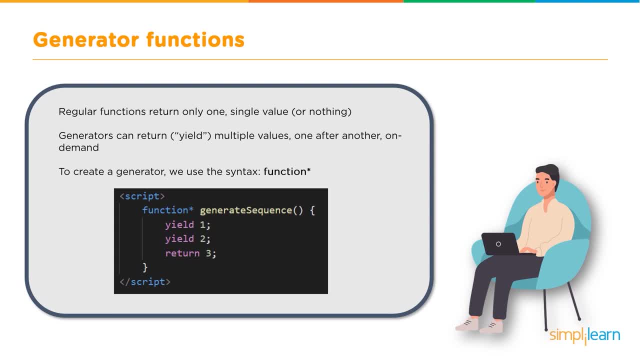 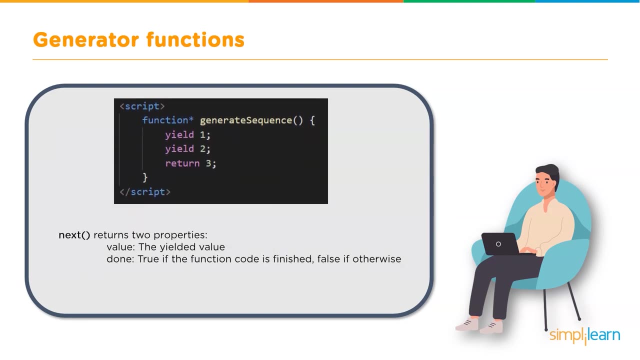 So here you can see that we have a function followed by asterisk and we've created a function called generator sequence. So here you can see, we have the asterisk after the keyword function followed by the name of the function. right, But the main method of a generator function 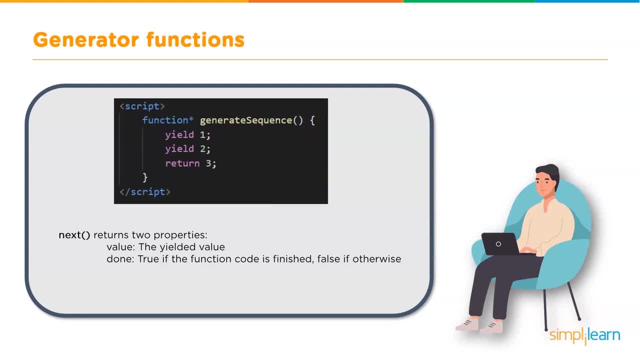 is the next method. When this method is called, it basically runs the execution until the nearest yield value, All right, or the nearest yield statement. Then the function execution pauses and the yielded value is returned to the outer code. All right, So the result of the next method. 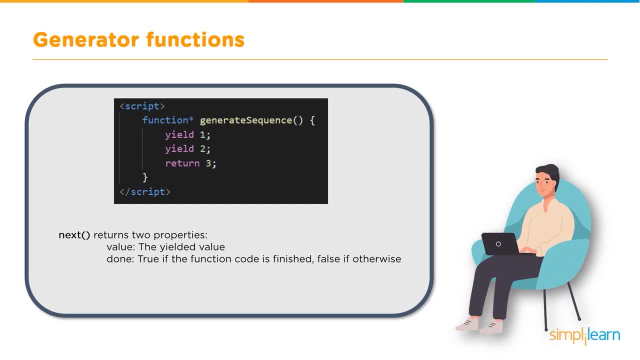 is always an object with two properties. It has a value property, which is basically the yielded value, And then it has a done property, which displays true if the function code is finished, or false if it's otherwise. So let me show its execution for a clearer understanding. 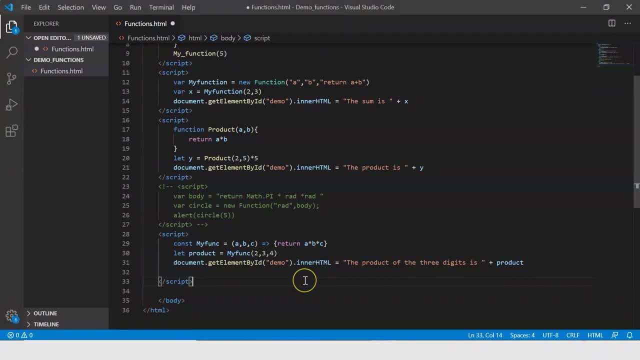 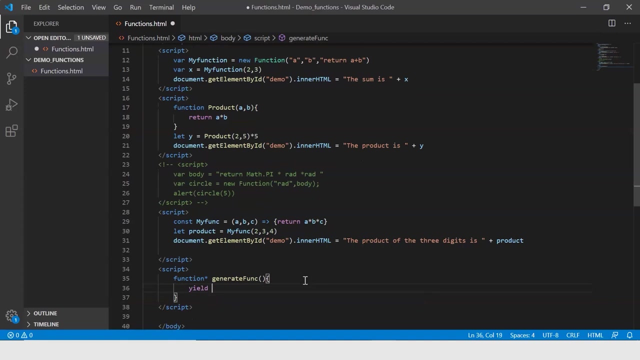 So let's go back to our VS Code And here let's create the generator function. Let's say: function, function, asterisk, generate function, all right Now, within which I make use of the keyword yield and I say yield one first. 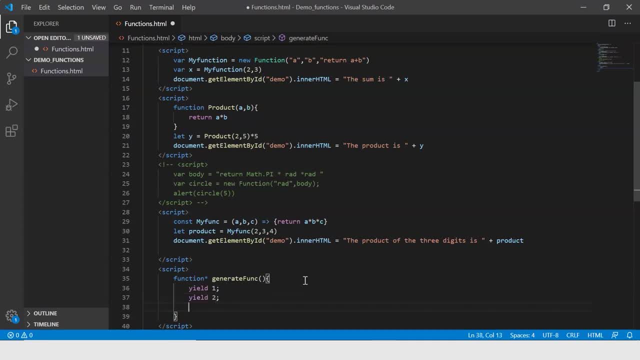 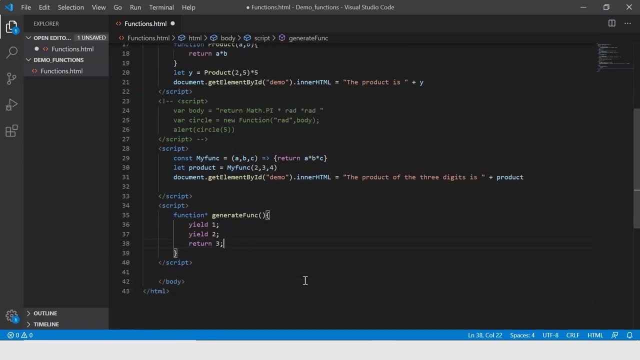 followed by yield two. And then, finally, I make use of return, which indicates the termination, So I say return three. all right, Now let me make use of a variable, say generator, and assign it to the generator function, That is, generate func. 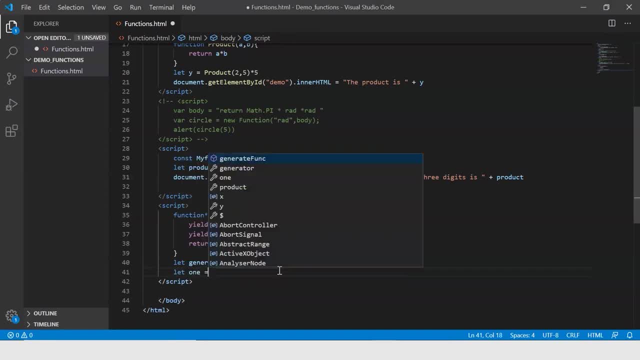 And now I create another variable, say one which will basically return the value when I call the next function. So here I say: generator dot next, Okay, So whatever generator dot next returns, it's stored in one. So to display the message I say alert. 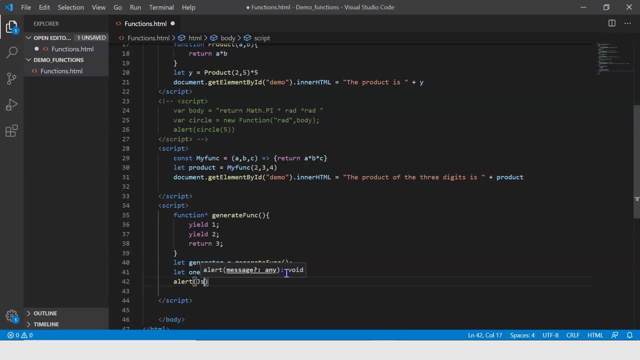 And now I'm gonna make use of a method called jsonstringify. all right, So, basically, this method converts a JavaScript object or a value to a JSON string, all right, So within which I'm gonna say one, That is this, all right. 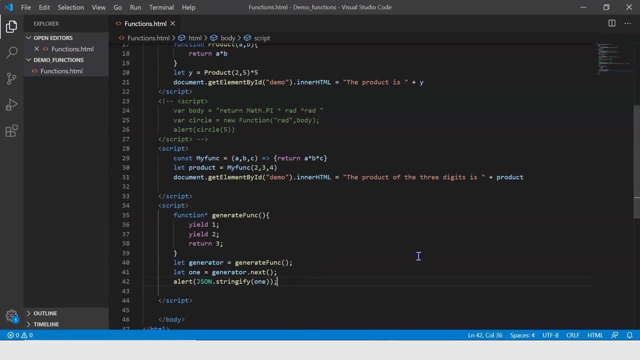 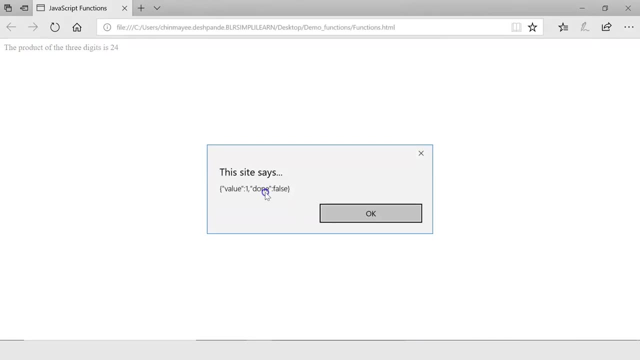 So now let me save this and execute it. Let me refresh the page and there you go. Here it returns two properties, that is, value and done. It says value is one and done is false. right, It is false because we haven't reached. 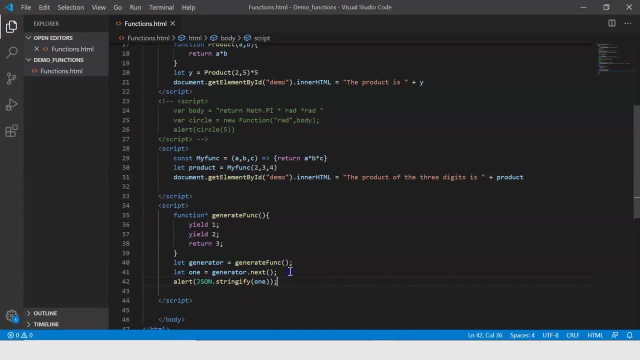 the return statement yet. So what we can do is to display the rest. let me just copy these and display it one by one. So here let's do this, and here let me say two, and this is three. Then we copy this. 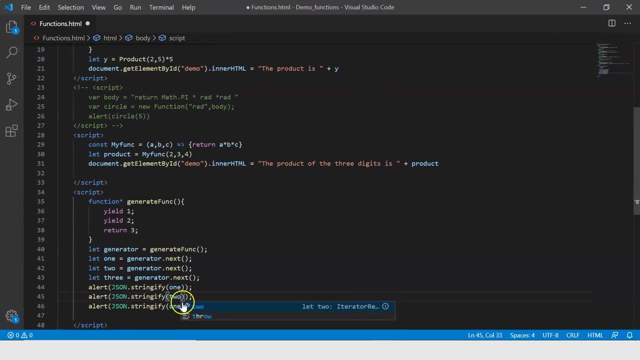 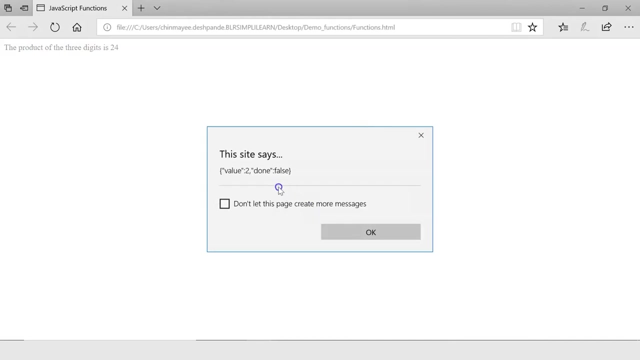 Okay, here I say two and then I say three. All right, so let me save this and then execute it. So when I look at the configuration, these are the locations. When I refresh the page, it says 1 and false, after which again it says 2 and false. 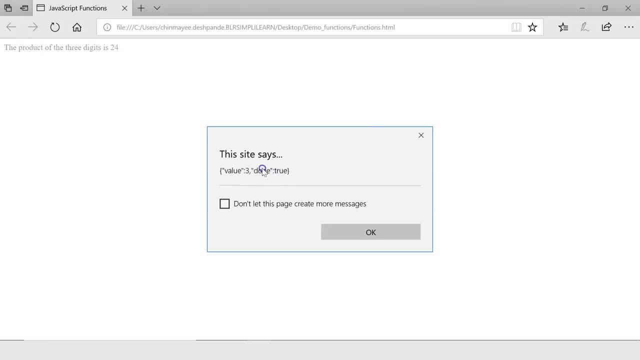 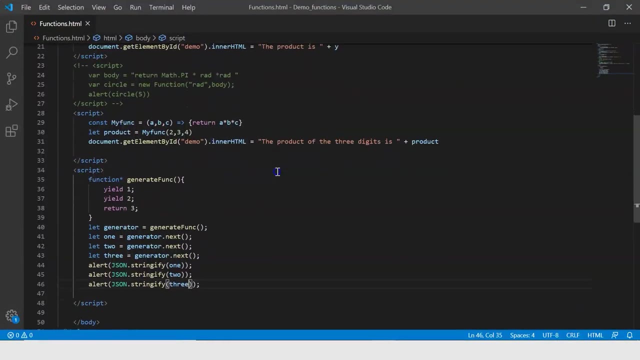 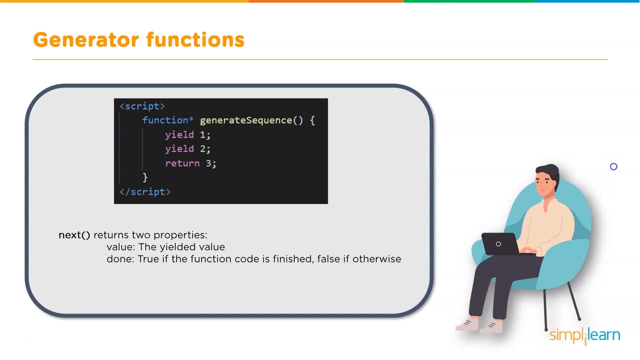 And finally, when it displays 3,, it returns true for the done property. That means we've reached the end of the function definition. So this is how you make use of a generator function. Now let's move on to our last topic, that is, predefined functions. 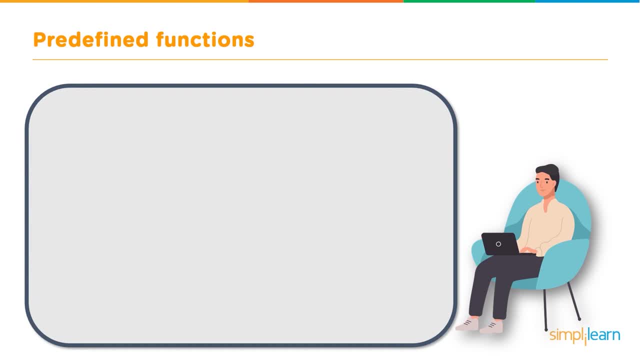 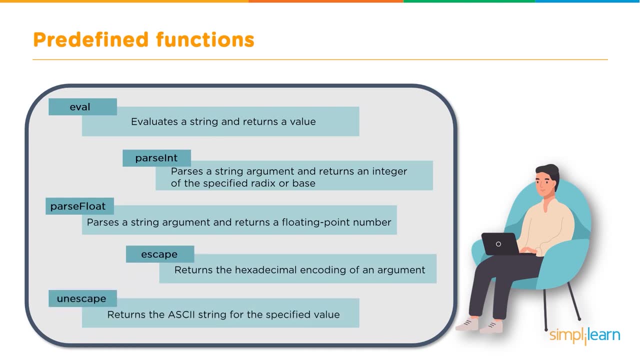 Now JavaScript has many built-in functions. alright, Now here are a few of them. We have eval, parseInt, parseFloat, escape and unescape. Now let's go through one by one. Alright, first up is eval. Now this basically evaluates a string and returns a value. alright, 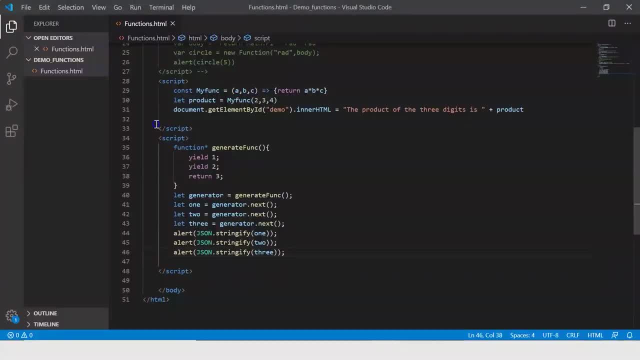 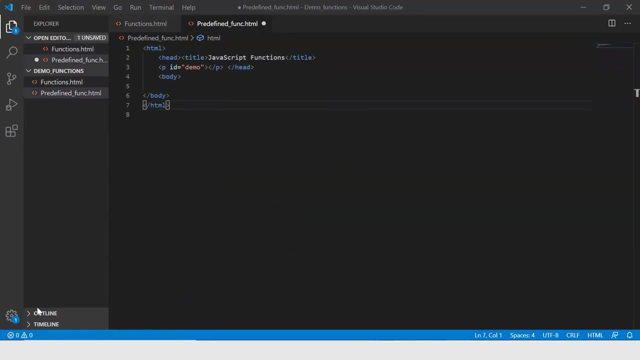 So, to help you understand this better, let me go back to our VS Code. And now let me just create another file and let me call it predefined, And I've just copied the initial code. alright, So for eval, the syntax is eval, within which I say expression: alright, 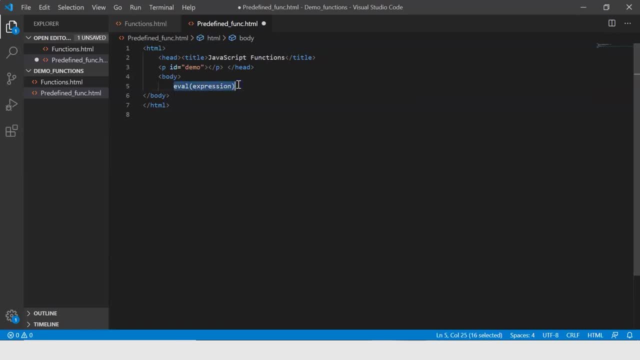 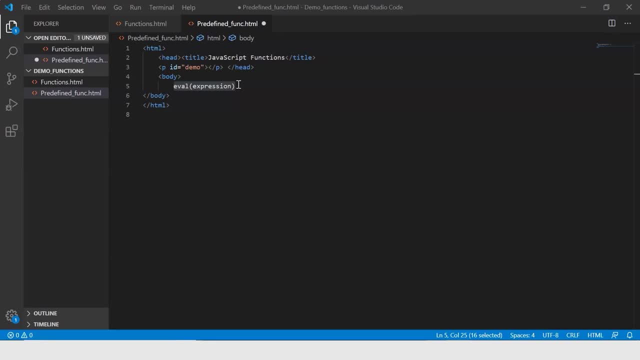 And if the result is not a string, the result is just returned. So now let's say that the result is a string. it is taken to be a JavaScript program and evaluated. So let me show you how it's done. So first let's create three variables. alright, 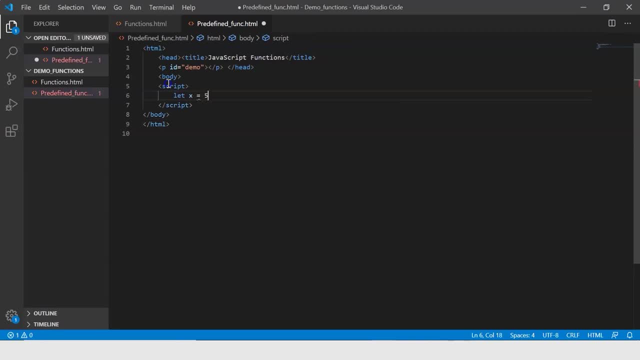 Let's call them x and initialize it to 5,, then y with 6, and then let z be 7,. alright, Now let's just displace the result. Alright, So the expression gets evaluated on the console. So let's say: consolelog eval of, let me say, x plus y. alright, 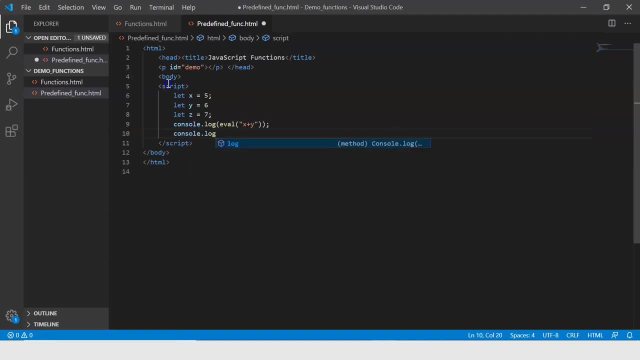 After which I again say: consolelog of eval of z. Here, since the expression is a string, this gets evaluated, And here, since it's not a string, it just returns the value z. So we have to try and approximate it to where z is. that's what we have to do. 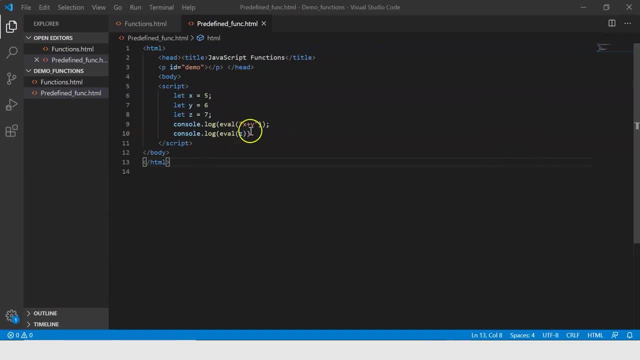 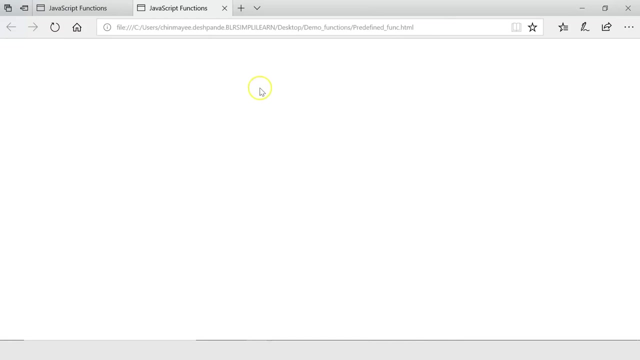 So first we've got to do an investigation. value z- And here, since it is not a string, it just returns the value of z. So let me save this and then execute it. Alright, so let me just check our console. There you go. 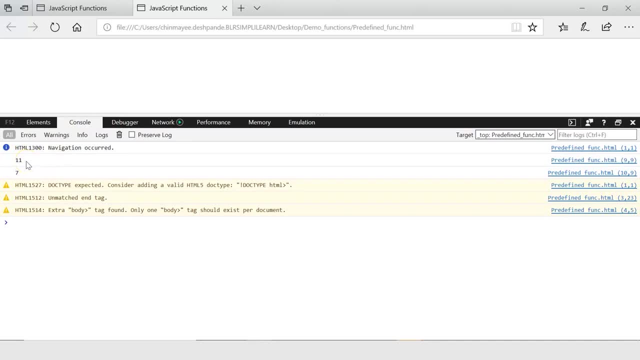 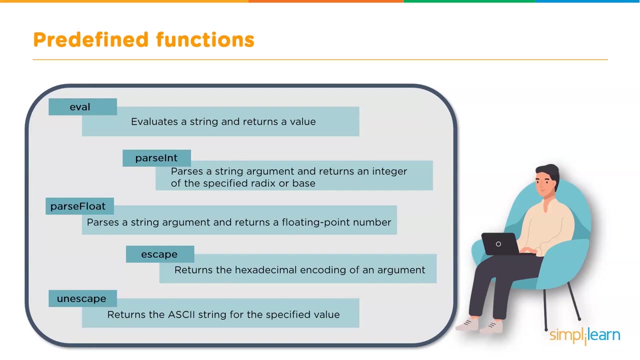 It evaluated the expression and added the two values, ie, x and y, and returned 11, while z is returned as it is. Alright, this is what eval does. Next up is parseInt. Now, as the name suggests, it parses a string argument and returns an.